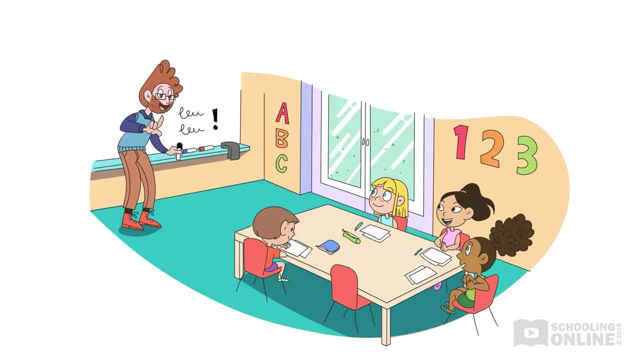 Holly, Molly and Polly are best friends At school. they have been learning some important ways to stay safe. Every Monday morning their teacher, Mr James, helps them learn what to do if they are ever in danger. Already they have learnt about swimming pool danger road. 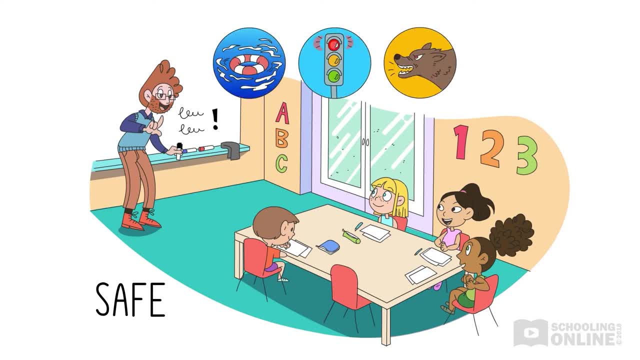 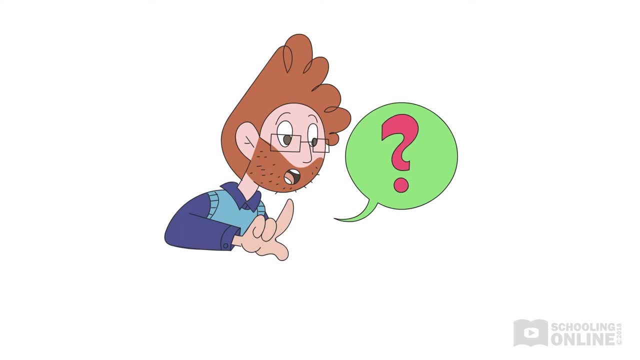 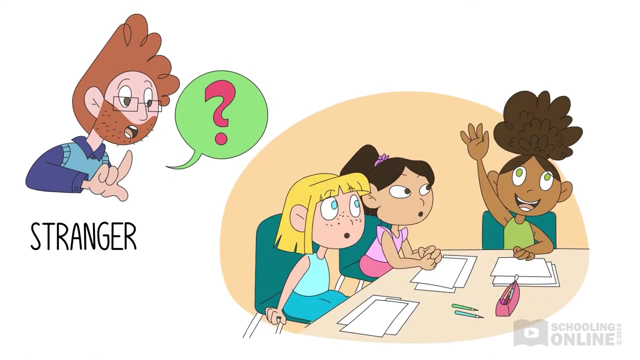 danger and what to do if a dog behaves dangerously. Today they are learning about stranger danger or how to keep away from dangerous strangers. First the teacher asks the children: Who is a stranger? Someone who looks strange, asks Polly. Sometimes strangers don't look strange at all. their teacher replies: 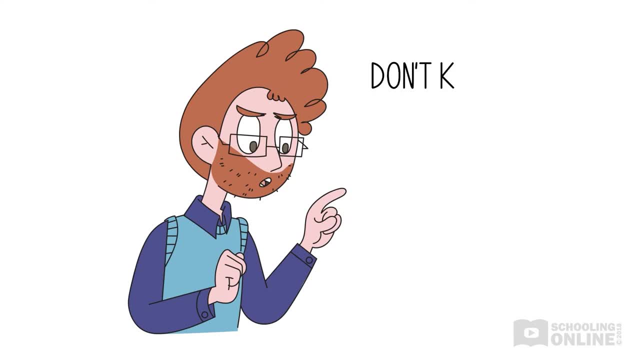 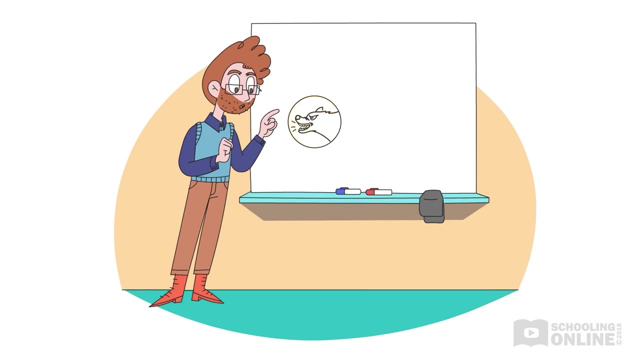 Actually a stranger is somebody you don't know. he says A stranger is someone you don't know. he repeats because it is important to know who a stranger is. You know what a dog looks like, so you can be on the lookout for dangerous ones. But 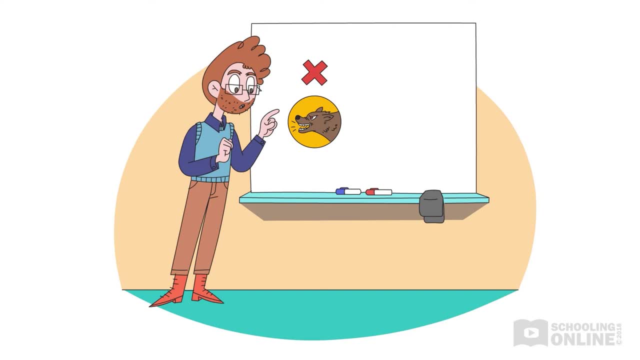 a stranger can look just like an ordinary person. It can be tricky because they don't always look dangerous. But if a stranger, someone you don't know, calls out and asks you to go over to them or go for a walk, you can say: 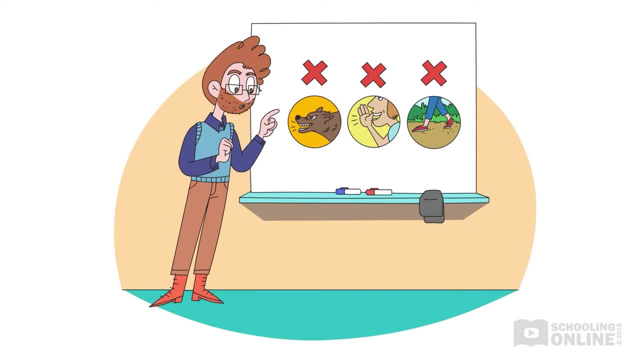 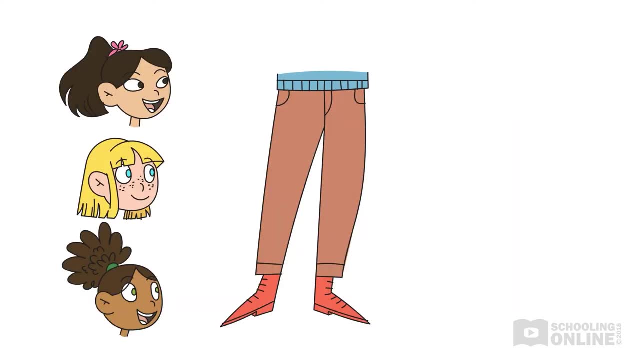 or get into a car. this means danger. Mr James chooses three people- Holly, Molly and Polly- to help him show the class what to do about stranger danger. First he asks Holly to show the class what to do if a stranger comes over and offers you lollies but says you have to come and get them from his car. 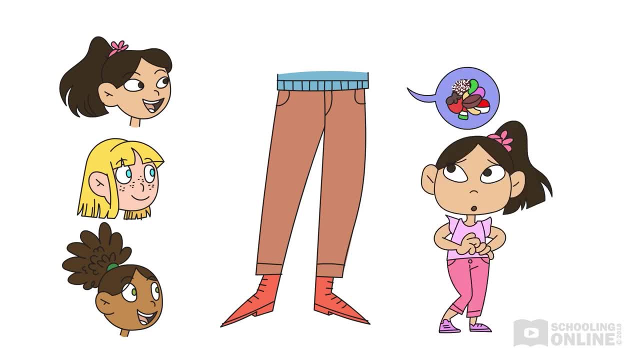 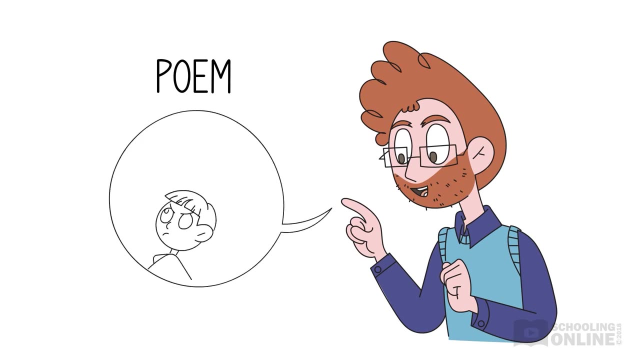 Mr James will pretend to be the stranger. Holly is a little bit nervous because she is not sure what to do. So before they start, Mr James teaches them a simple poem: If a stranger comes your way, do not stop, do not stay, do not speak or start to play.